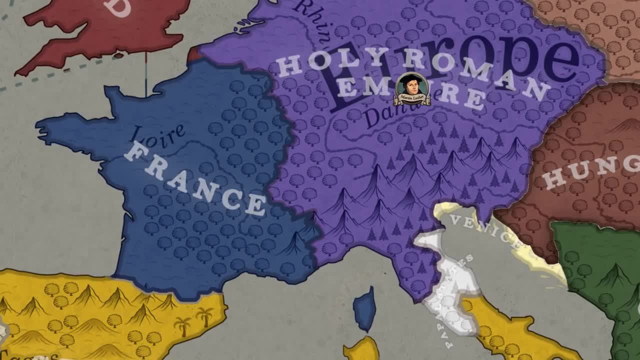 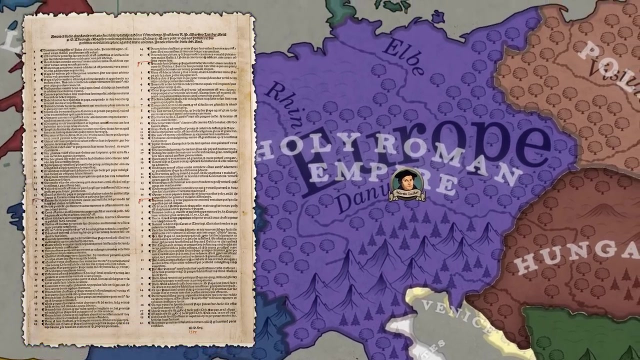 the making, and Martin Luther was not its only leader. While many view the start of the Protestant Reformation as having been in 1517, following the publication of Martin Luther's Theses, the actual date of its beginning is somewhat unclear. There were essentially three main 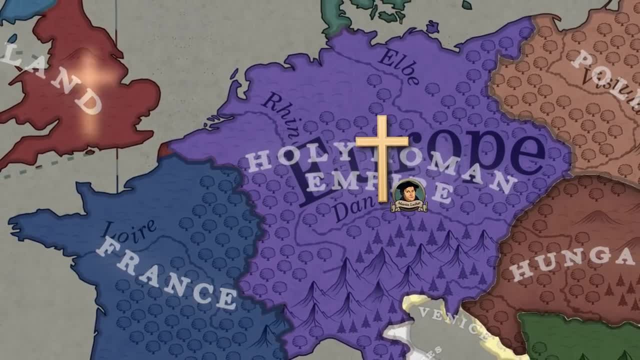 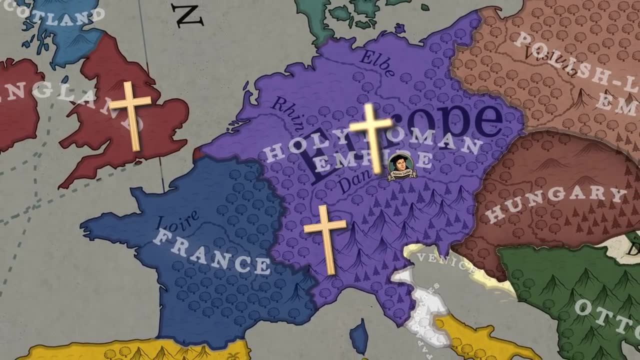 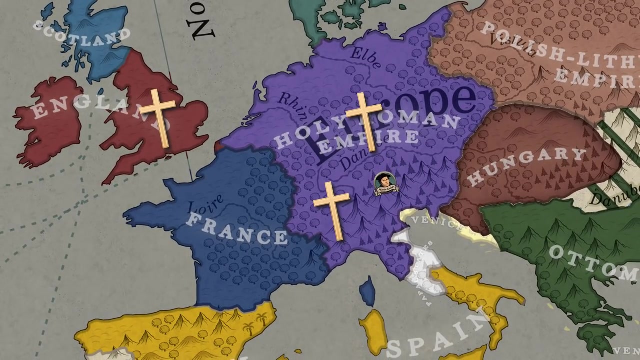 Reformation movements, one in Germany, one in England and one in Switzerland, with all of them occurring around the same time in the 16th century. The German Reformation led by Martin Luther is generally the movement that most people think of when the topic is. 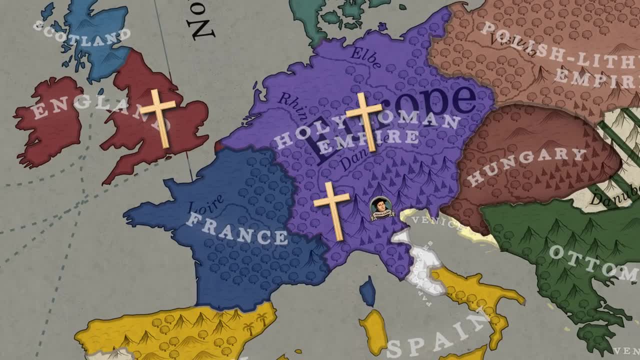 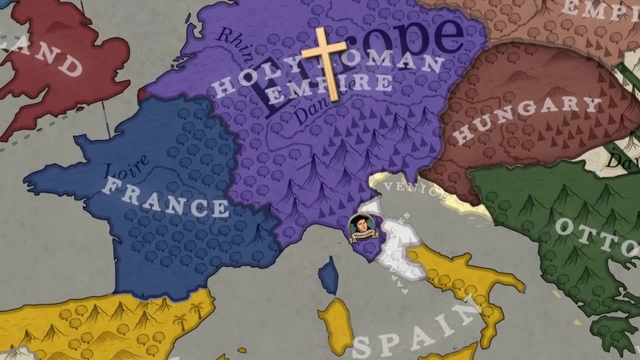 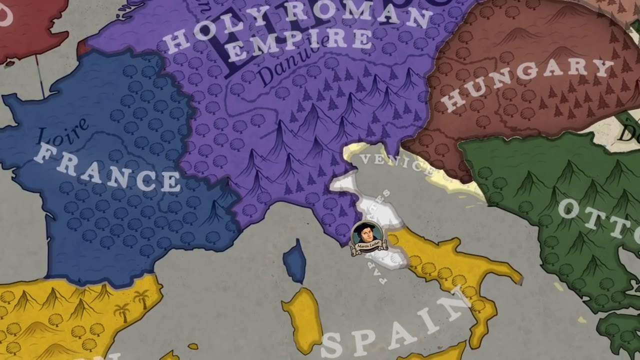 discussed. Martin Luther prior to the Reformation was actually a professor of theology and a priest During his time. as such, Luther was sent to represent the observant German Augustinian monasteries in Rome between the fall of 1510 and spring of 1511, where he came to notice a lack of 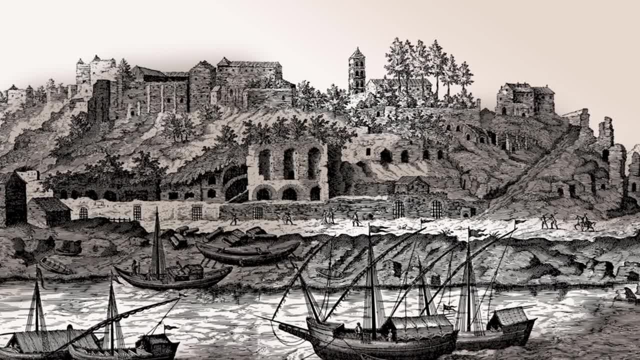 spirituality throughout Rome that left a lasting negative impression on him. This pessimistic view of the Church only worsened after Luther's death. Martin Luther was sent to represent the observant German Augustinian monasteries in Rome between the fall of 1510 and spring of 1511, where he came to notice a lasting negative impression on him. 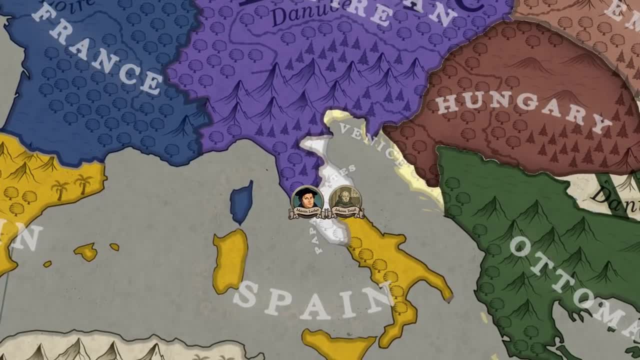 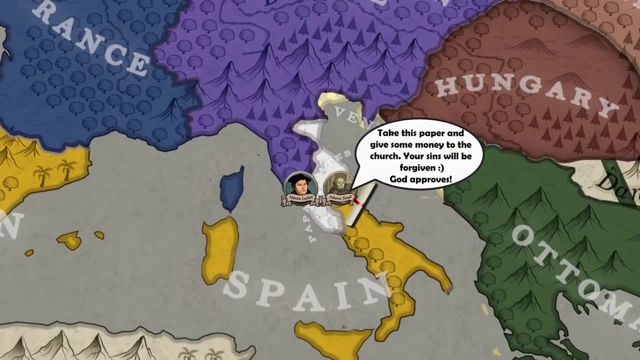 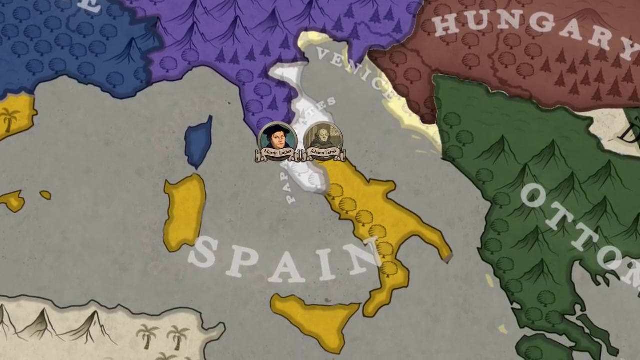 Martin Luther discovered a Dominican friar, Johann Tetzel, who preached that sins could be forgiven by the purchase of a letter of indulgence, approved by the Pope, allowing for one's soul to skip time in purgatory before entering heaven. The money from these indulgences was being put. 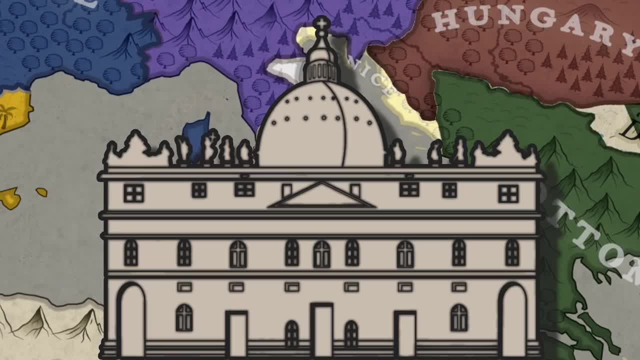 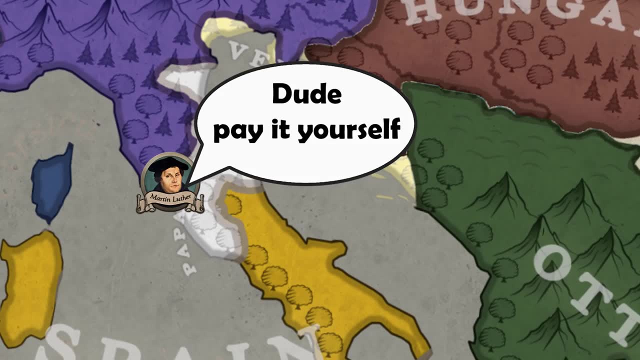 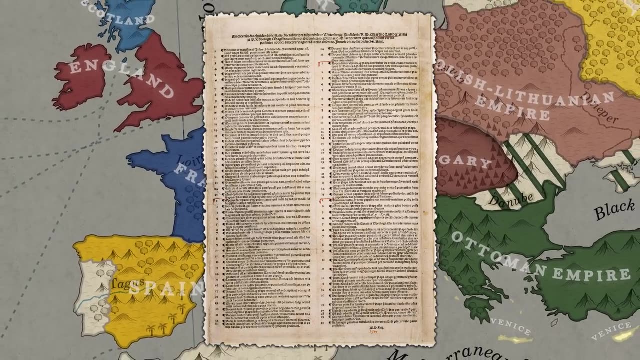 toward the rebuilding of St Peter's Basilica in Rome, which Luther bravely claimed should be paid for by the wealthy Pope himself. In response to this indulgence, Luther wrote his Ninety-Five Theses, which was supposed to inspire a debate about the. 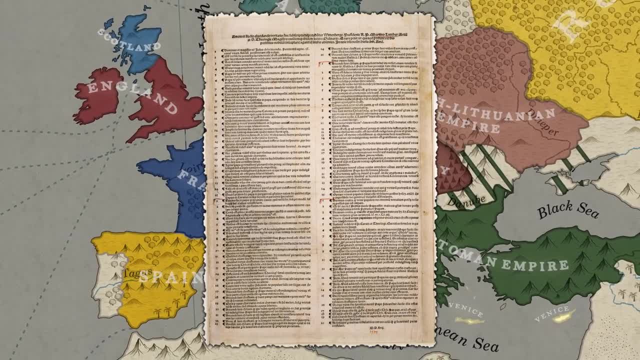 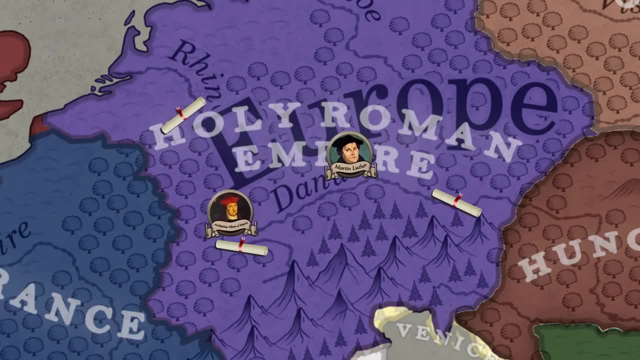 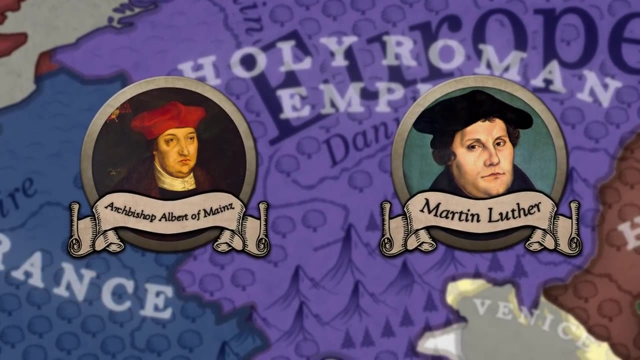 issuance of indulgences, with the assumption that his concerns would be heard and understood. Copies of the propositions were sent out to a few friends and to Archbishop Albert of Mainz, who was Tetzel's superior, accompanied by a request for the friar's preachings to 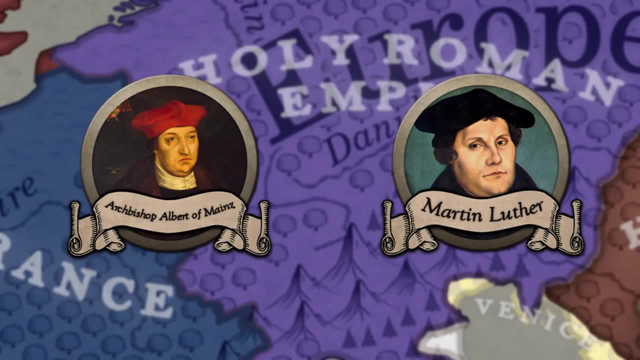 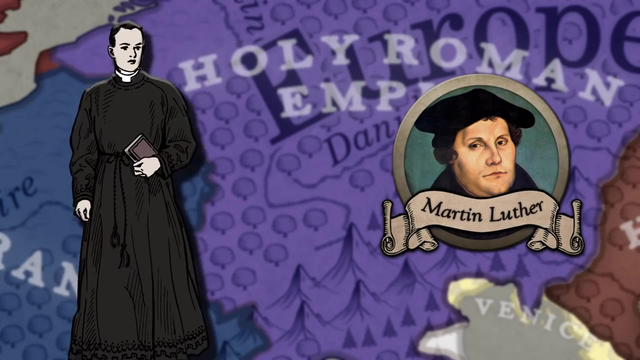 be stopped. Luther's grievances were not met with the reaction he anticipated, and his disapproval of the Church began to expand into growing theological disagreements. By 1518, Luther had come to believe that the view of the Church, which stated that salvation came, 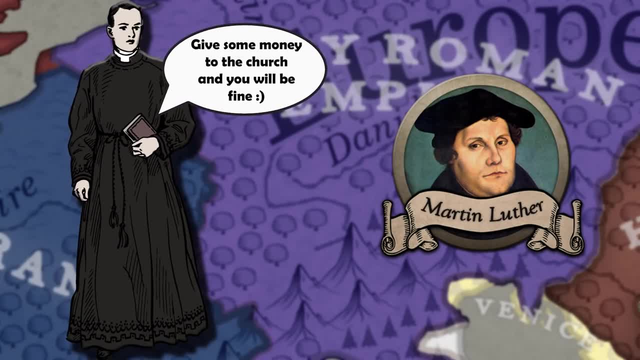 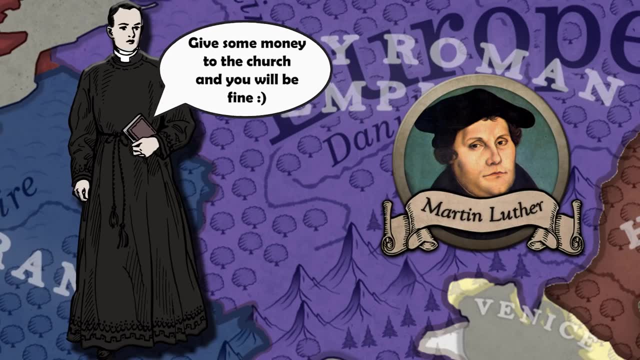 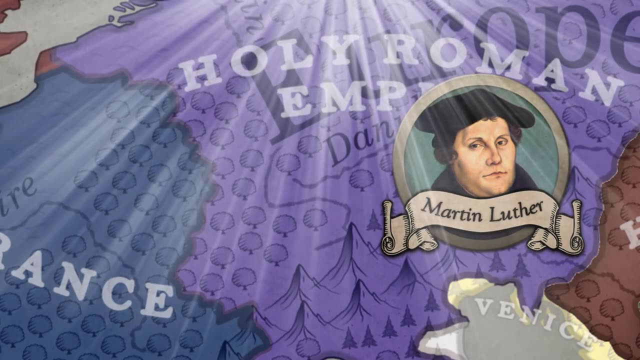 from both the grace of God, in addition to good works and human actions, to earn reconciliation was utterly false and that humans were unable to earn salvation. It was simply an act of God's forgiving grace. Furthermore, Luther came to the conclusion that the 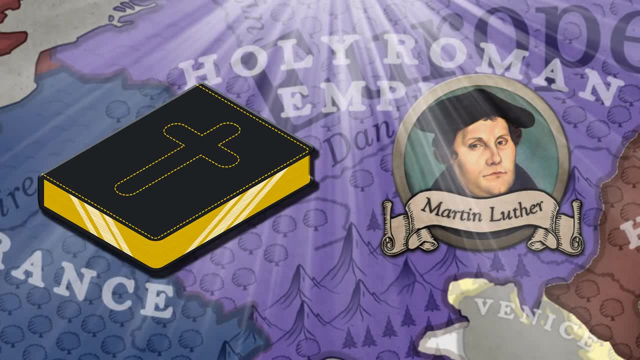 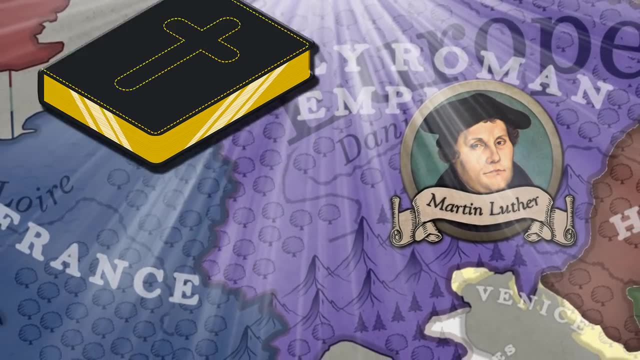 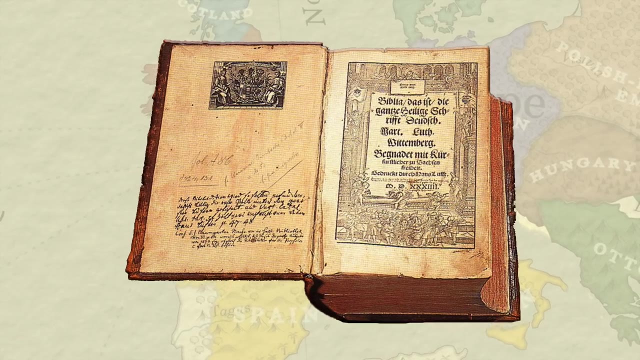 Bible itself should be viewed as the only reliable source of information and authority, as opposed to the teachings of the Church and the Pope having that role. Since the printing press had recently been discovered, this gave Luther a vast advantage, as new translations of the Bible could now be printed and provided to anyone with the ability to read, so that 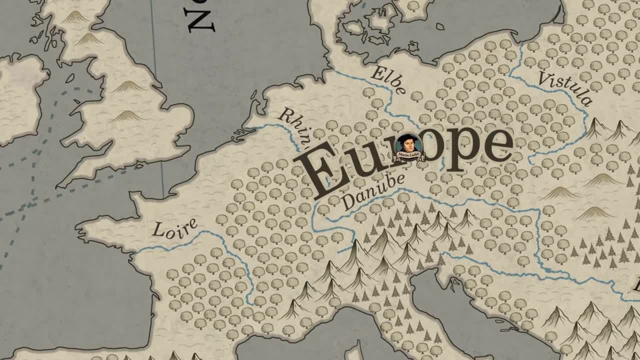 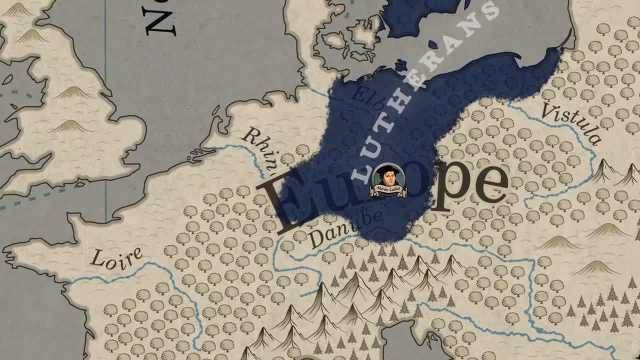 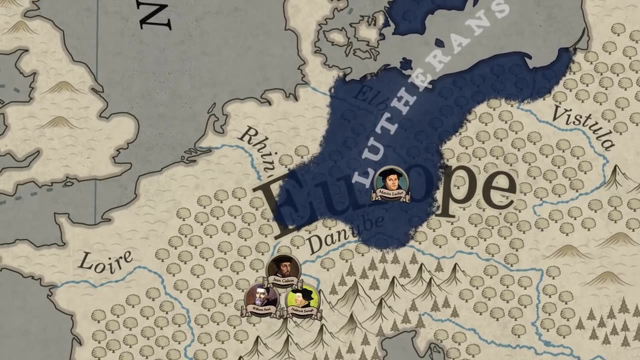 they could learn from the Bible themselves instead of relying on priests and other clergy members. In England, a reformation paralleling Luther's began around 1522, under the guidance of Holdrich Zwingli, William Farrell and later John Calvin. Zwingli, a priest, taught similar ideas to 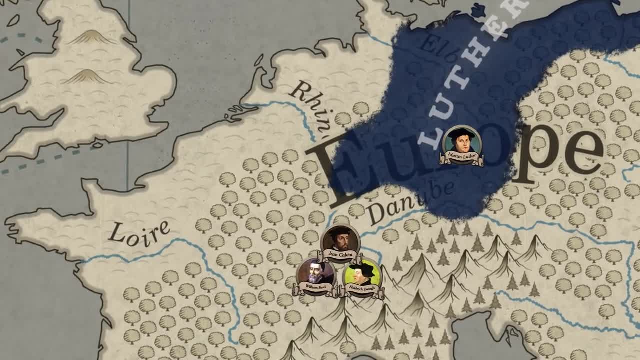 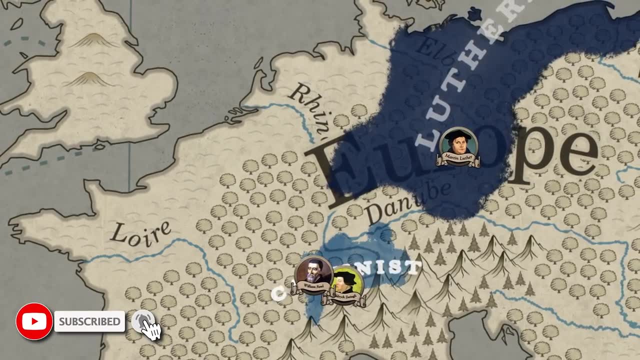 what Martin Luther was preaching in Germany, but on an even more radical level. Beginning in Zurich, Zwingli's movement quickly took a stronghold in the city, and by 1526, Farrell, a fellow reformer, had become a member of the Church. The church was then changed to: 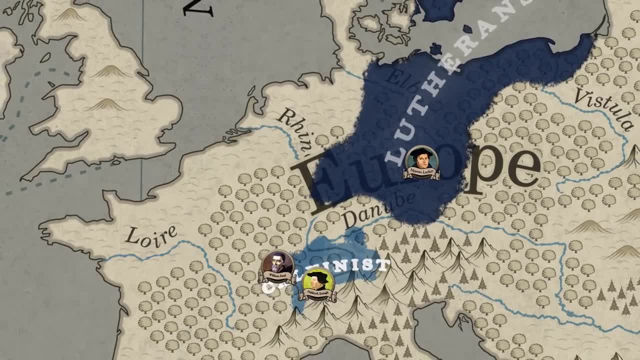 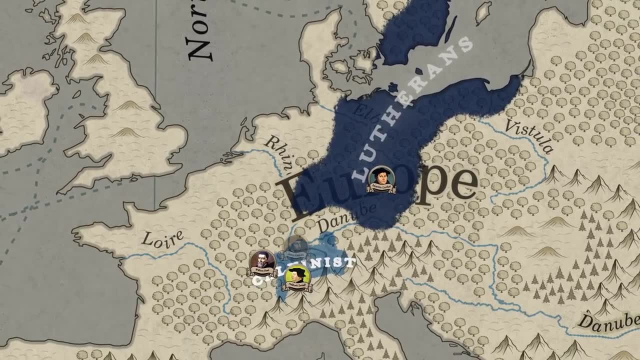 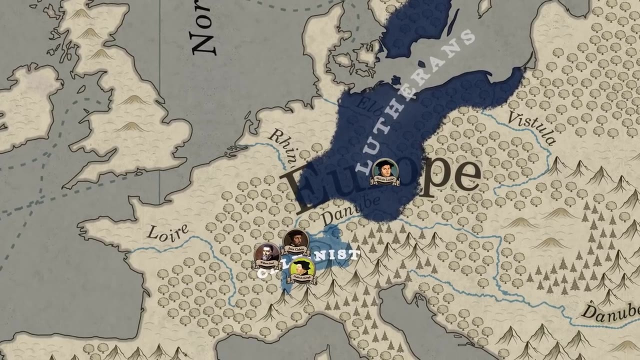 the Church of Geneva, where he began to assist him in spreading the message to the French-speaking parts of Switzerland, giving sermons in different cities, including Geneva. In 1536, Farrell met John Calvin, who authored the Institutes of the Christian Religion Doctrine and would 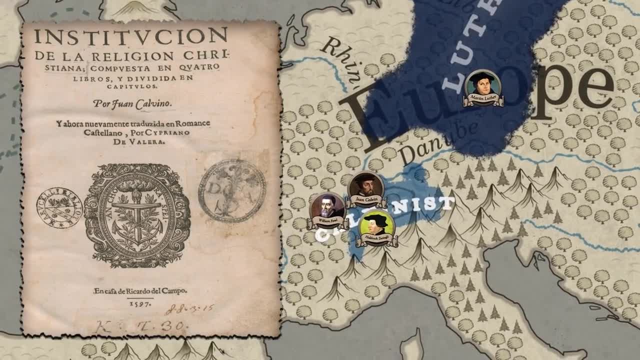 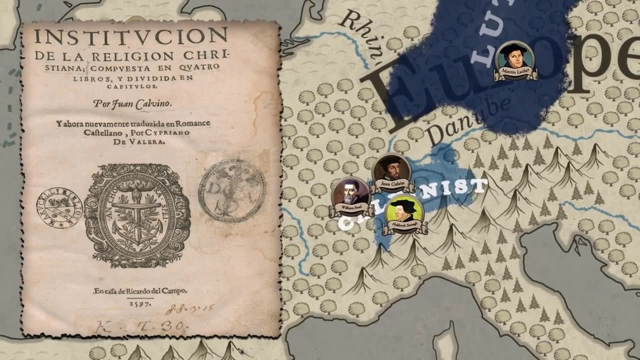 help Farrell to organize the reformed Church of Geneva. Additionally, Martin Luther was not the only reformer to translate the Bible into vernacular for the masses to read themselves, as the Swiss were the only ones to read the Bible themselves. as the Swiss were the only. to read the Bible themselves, as the Swiss were the only ones to read the Bible themselves. as the Swiss were the only ones to read the Bible themselves. as the Swiss were the only to read the Bible themselves. as the Swiss were the only ones to read the Bible themselves. 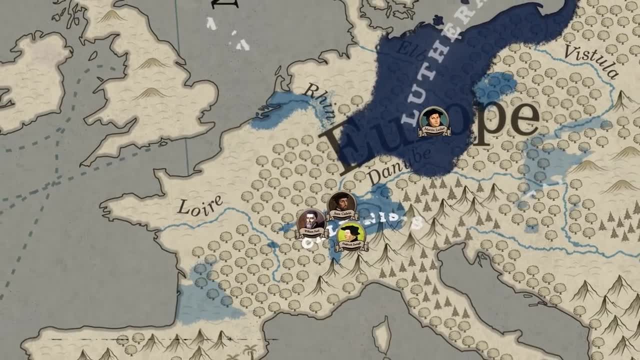 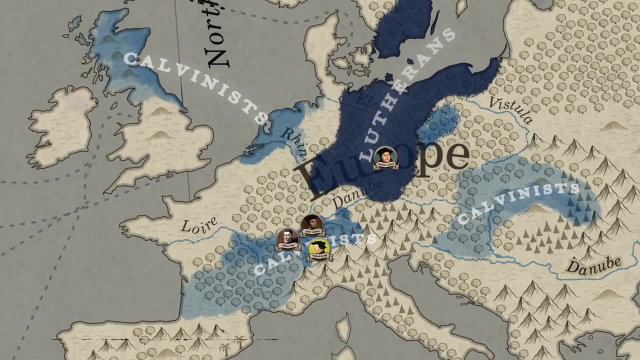 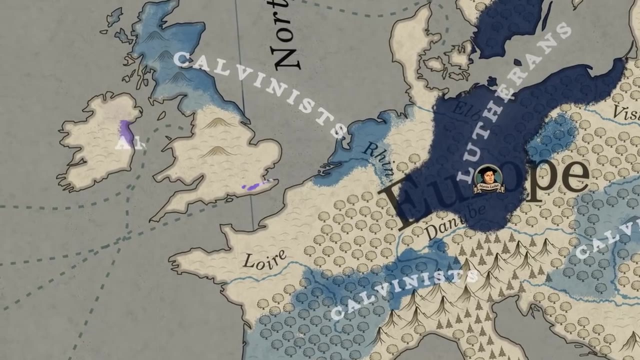 and so bothетеRWμέTheedis всethe inst the same. The reformation also spread rapidly in Switzerland, and Calvin's work reached as far as Scotland to the west and Transylvania to the east, As both Calvmizing and Lutheranism. 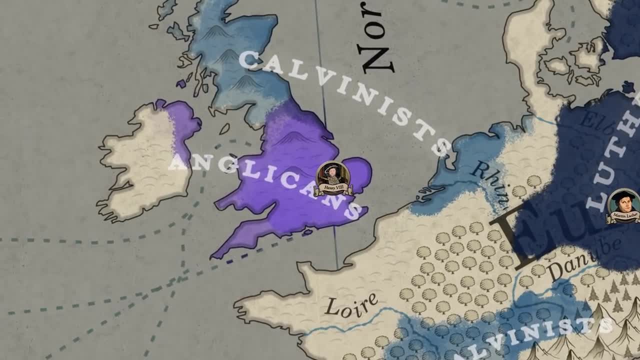 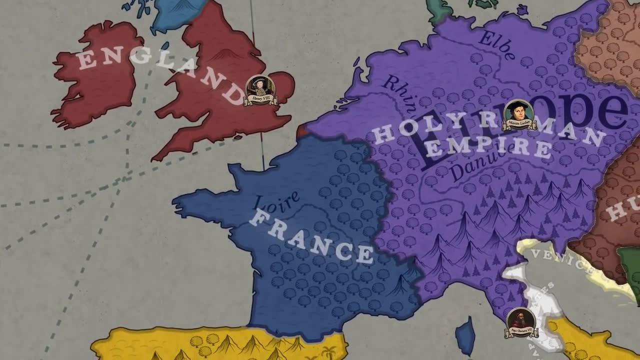 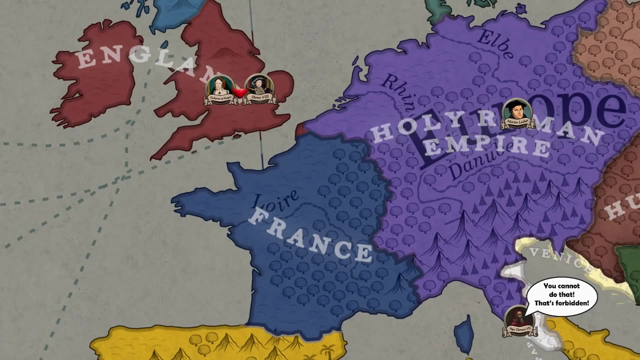 gained traction throughout Europe, England fell into its own reformation. In the far west, King Henry VIII prompted the third simultaneous reformation for both religious and political. Unfortunately, the monarch was outraged by Pope Clement VII's denial of an annualment for Henry's marriage to Catherine of Argonne. 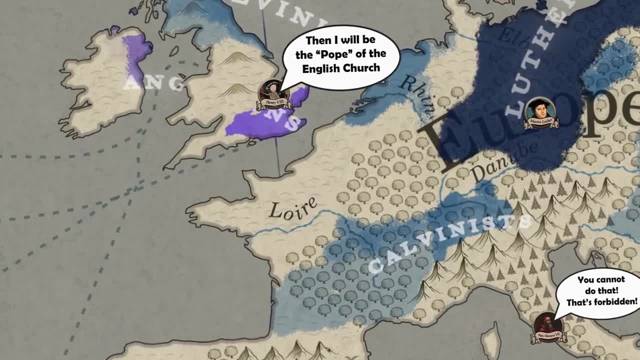 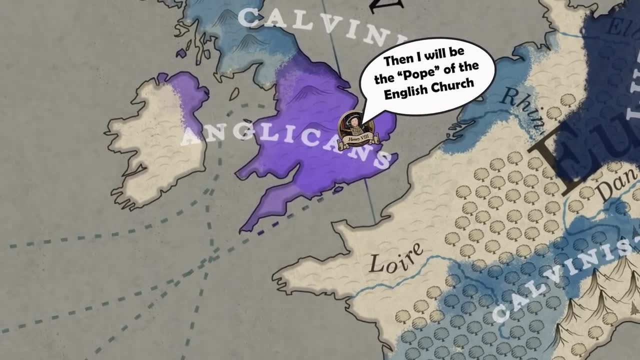 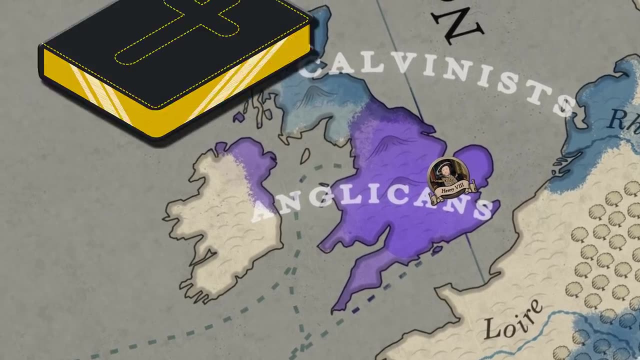 In 1534, the English king declared that he should, from then on, be the only final authority on all matters within the English Church, thereby establishing the Anglican Church and the start of a new Reformation movement. King Henry also insisted that the Bible be made available for the people, demanding that 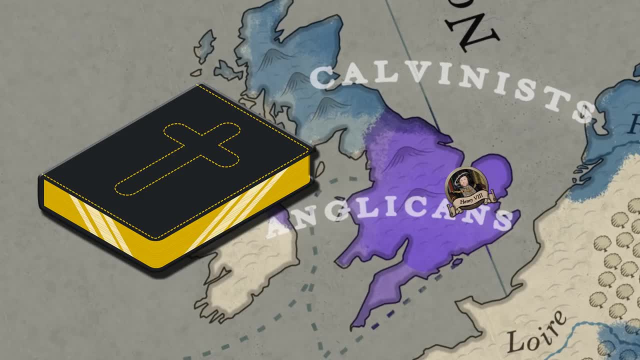 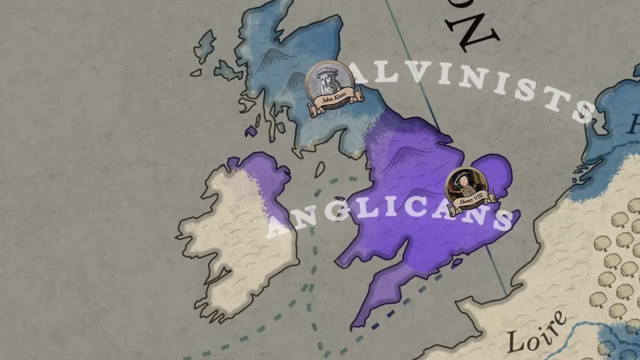 every parish obtain a copy, and additionally requiring that liturgy be prepared in English. Paralleling Henry's changes, Scotland also joined the reforms thanks to the inspiration John Knox received from John Calvin. back in Switzerland, Knox now formed the Presbyterian branch of Protestantism. 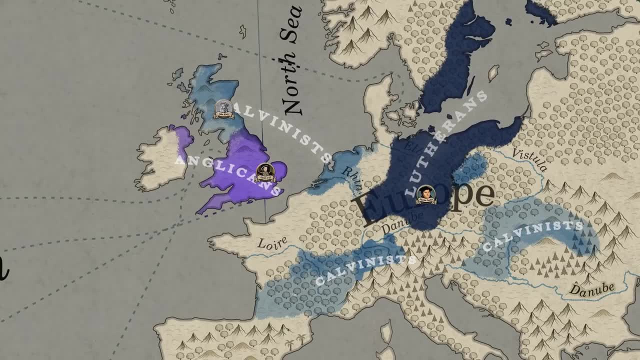 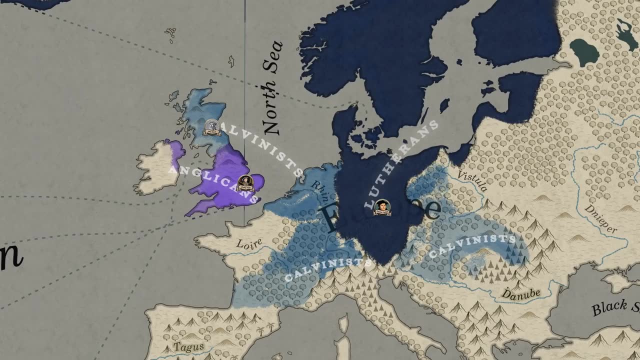 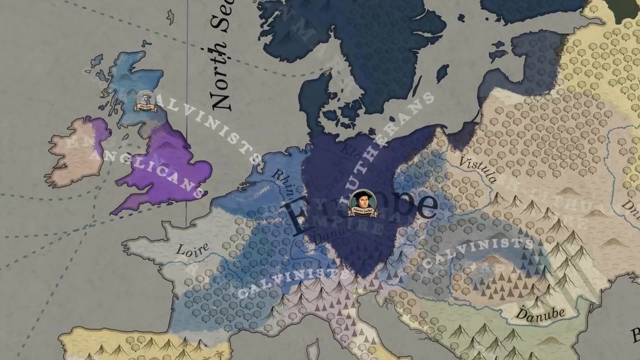 Eventually, though shamefully late, the Catholic Church formulated a systematic response to the growing Protestant Reformation in the form of what is simply called the Counter-Reformation. Although some steps were taken to address the reformers earlier on, such as the excommunication, 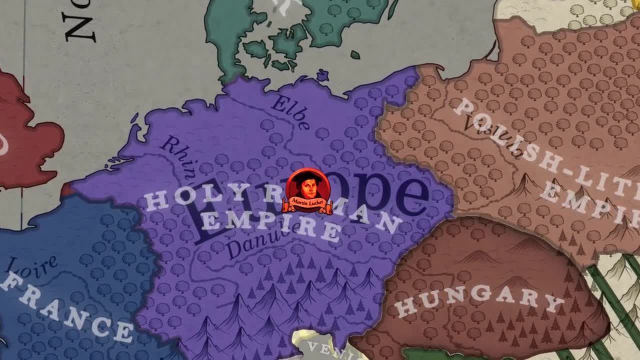 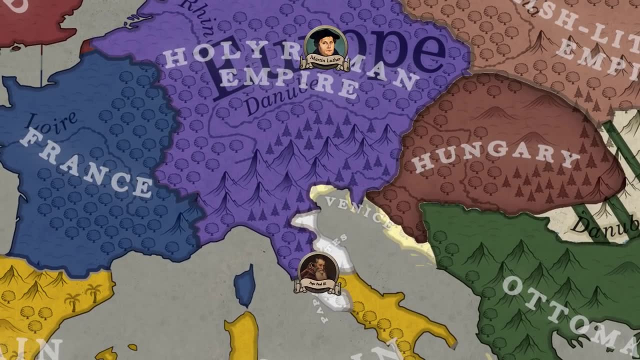 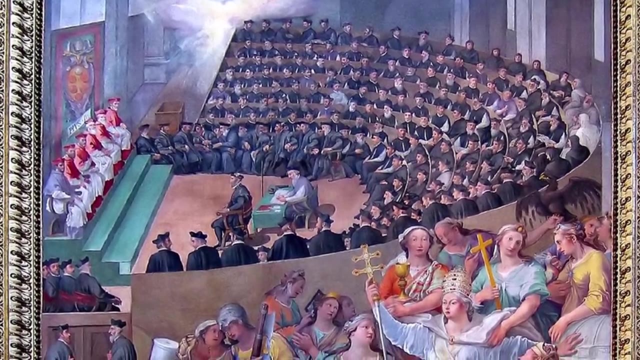 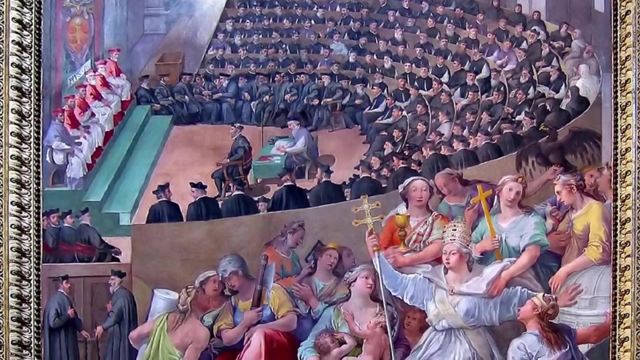 of Martin Luther back in 1521, the Catholic Church as a whole failed to do much at the start. The first major move taken by the Church was under Pope Paul III, who called for the Council of Trent in 1545.. The three-part series of councils held between 1545 through 1563, not only addressed the 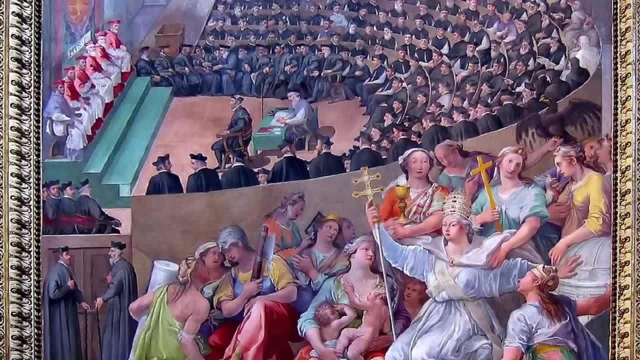 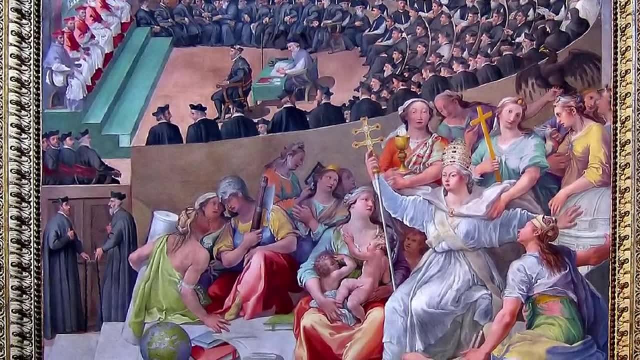 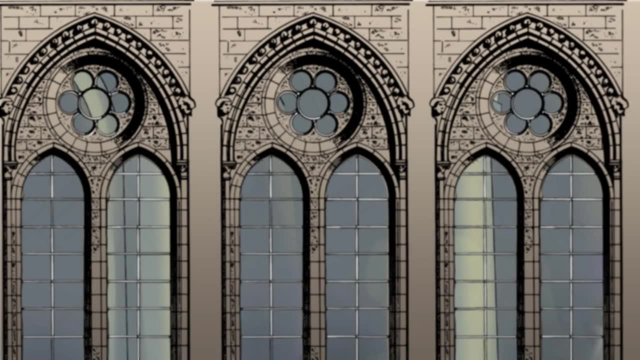 challenging of Catholic doctrine by the Protestants, but also established decrees of self-reform. In the first council, the bishops in attendance were divided as to whether full-out reform was needed or simply a clarification of Catholic doctrine. Many issues were discussed, such as the Creed of Nicaea and Constantinople, which was confirmed. 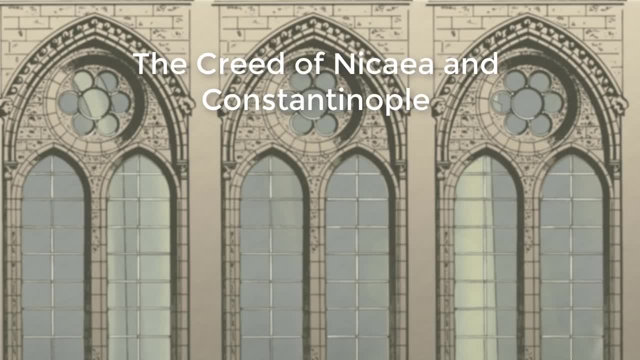 as the foundation of the Catholic faith, the number of sacraments, which should be seven, tradition, which was accepted as a source of faith, as well as other subjects that had been challenged by Martin Luther in particular, which subsequently led to the decision to. 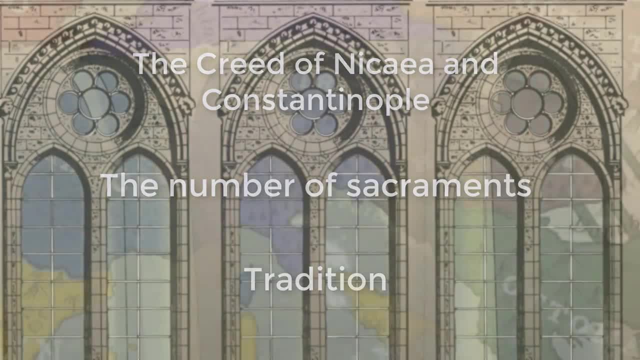 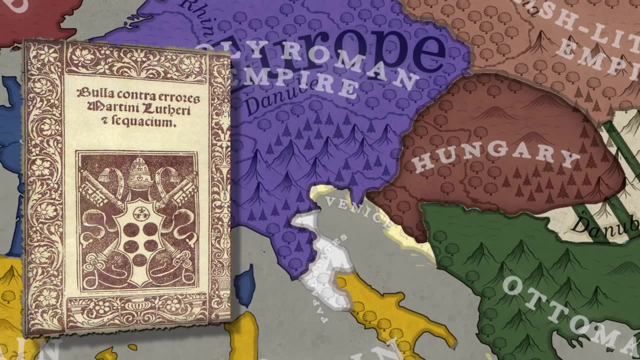 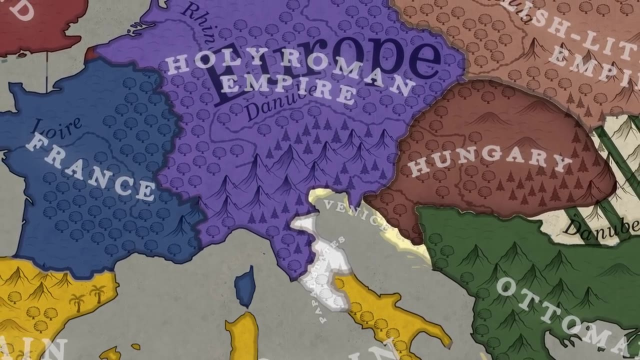 formally deny the reformers' idea that humans had no ability to earn salvation through behavior such as good works. Political discord put the progress of the council on hold until the next period of talks began in 1551.. As the second part started, a growing number of Protestants, mainly from Germany, began. 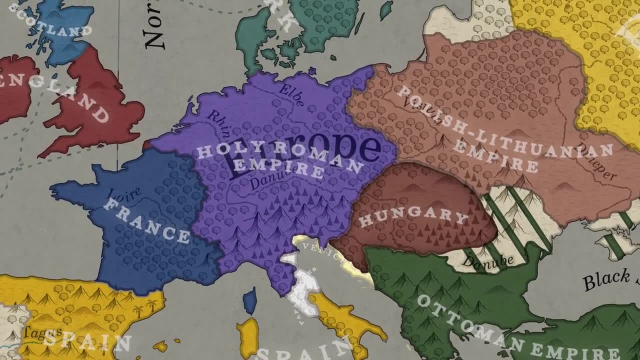 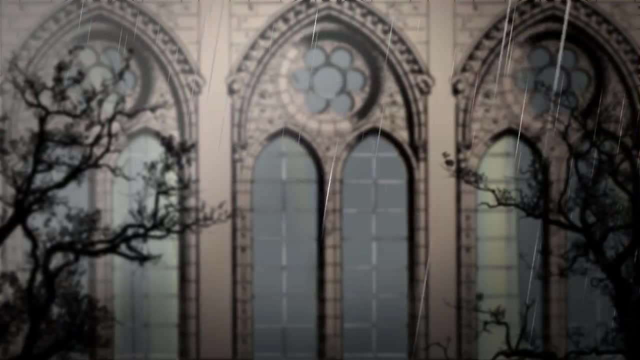 to assist upon a re-evaluation of what had been decided upon by the council back in 1545. But nothing of the sort was done and the council continued on. This time, one of the main subjects of the council was the Council of Trent. 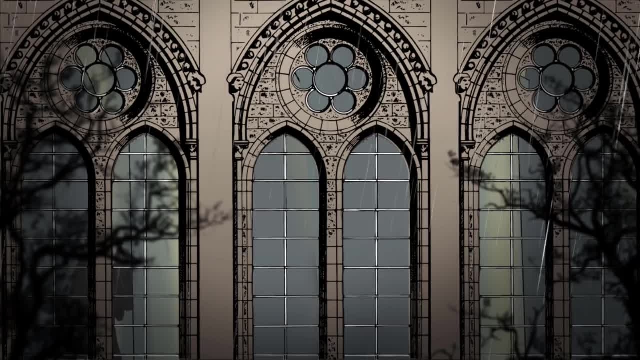 The Council of Trent was one of the main subjects of the Council of Trent. The Council of Trent was one of the main subjects of the Council of Trent. The Council of Trent was one of the main subjects of the Council of Trent. One of the major issues addressed was the sacrament of the Eucharist, which the Catholic 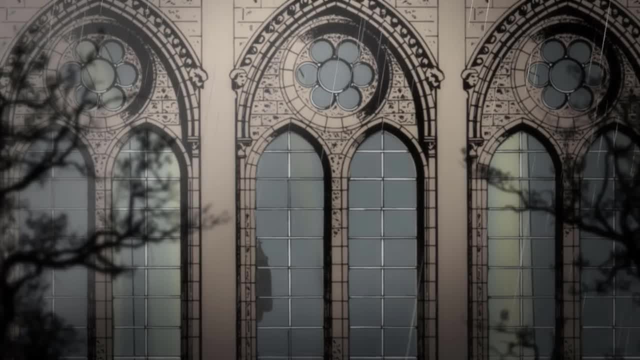 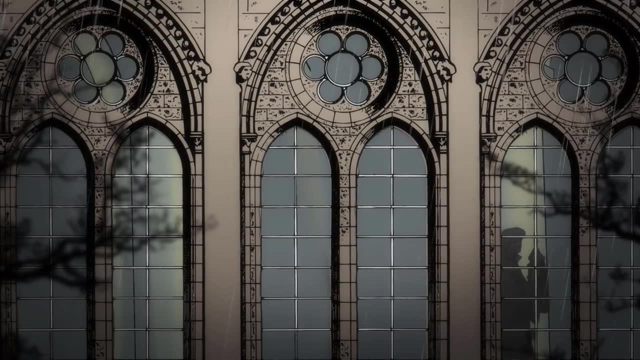 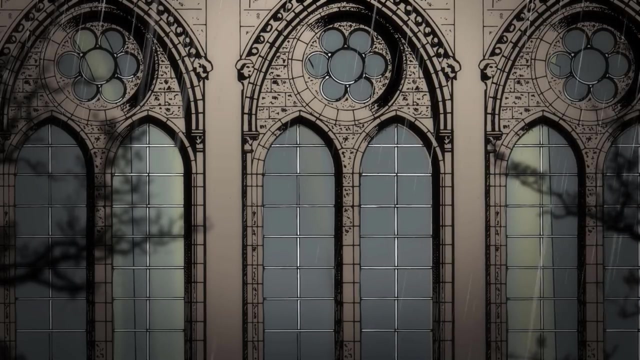 Church confirmed to include that the bread and wine were believed to truly transform into the body and blood of Christ, although not in appearance. This assertion was, of course, in direct contradiction to the reformists, which came as no surprise. Further doctrine, despite the many disconcertingί identities, was solidified before the council. 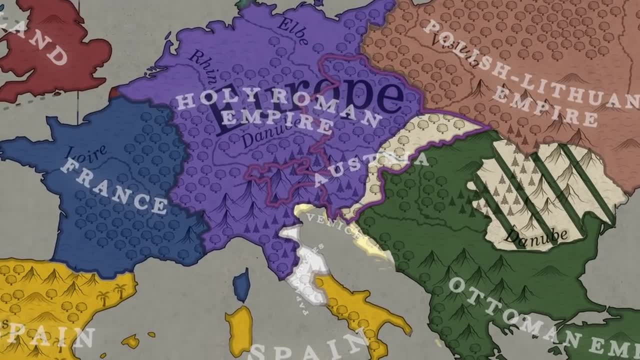 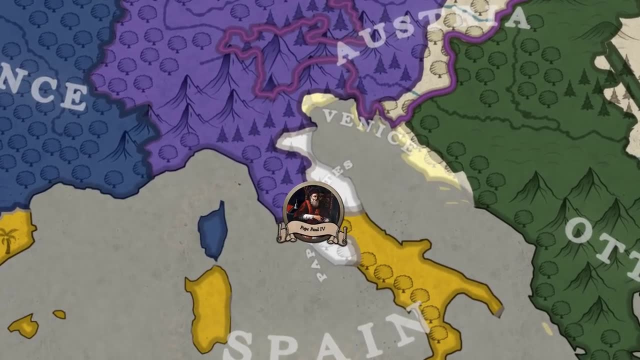 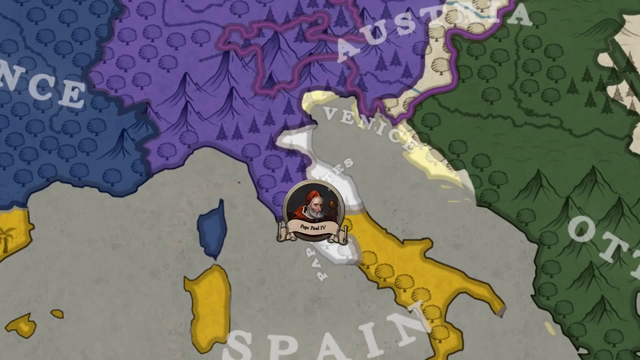 was interrupted by political disputes. yet again, when this mouse was closed before visiting, the Council again took over. the whole concept of the council came under serious doubt due to his direct opposition to the notion. Finally, in 1562, Pope Pius IV decided to reinstate the council. 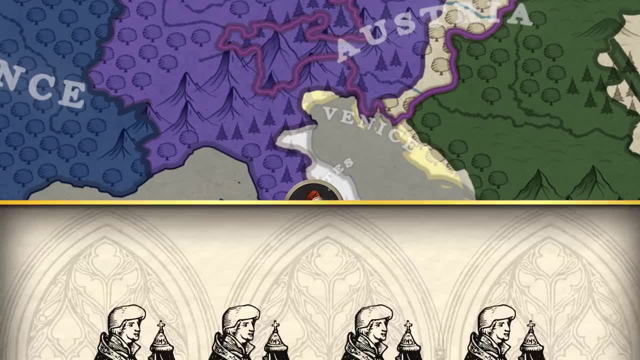 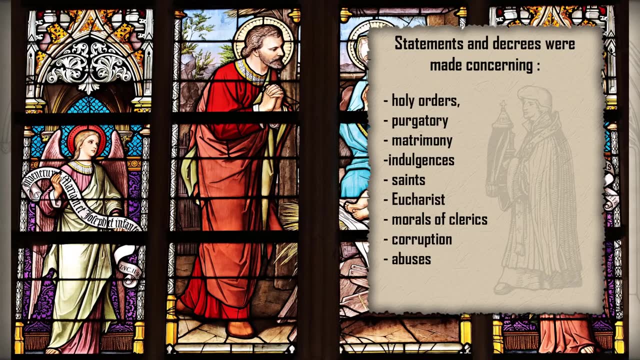 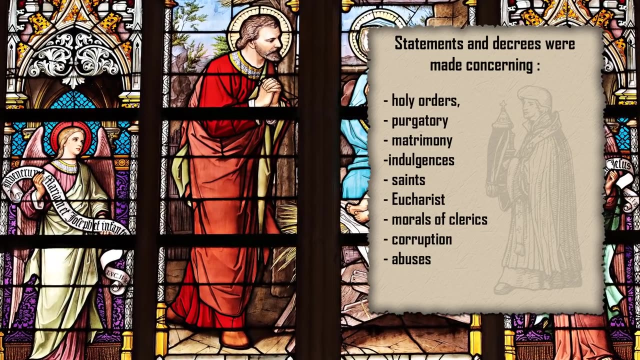 and the bishops regathered During the last leg of the meetings. updated statements and decrees were made concerning mass holy orders, purgatory, matrimony, indulgences, saints and again more details concerning Eucharist. Reforms were also made for the morals of clerics. 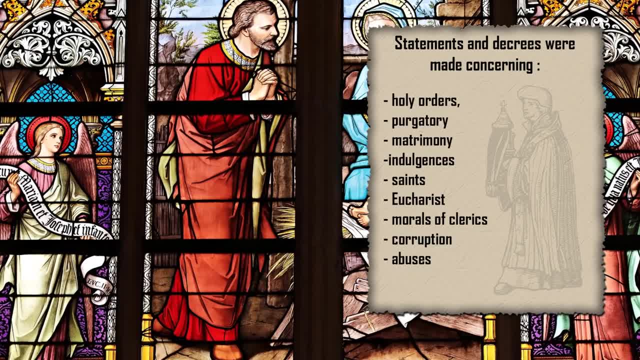 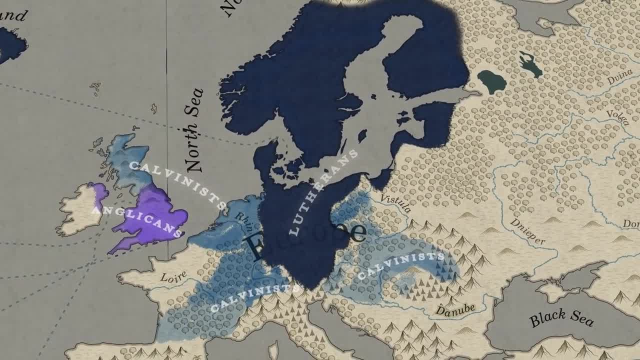 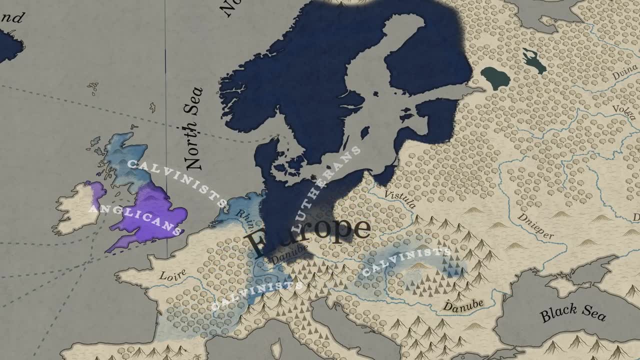 and much of the corruption and abuses that had inspired the Protestant Reformation, such as the clerical overspending and favoritism within appointments made to the church office, were soon resolved, allowing the Catholic Church to regain a large amount of its support throughout Europe. Still, it was too late to reverse the break within the Western Church. 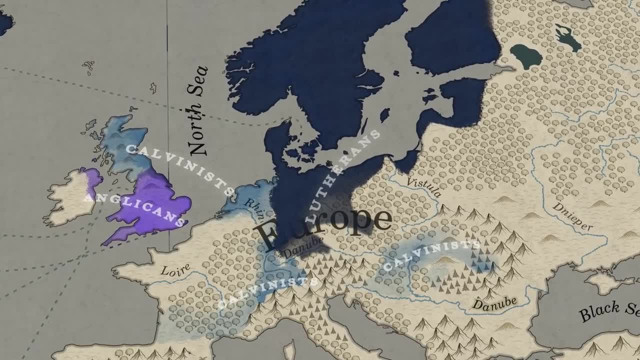 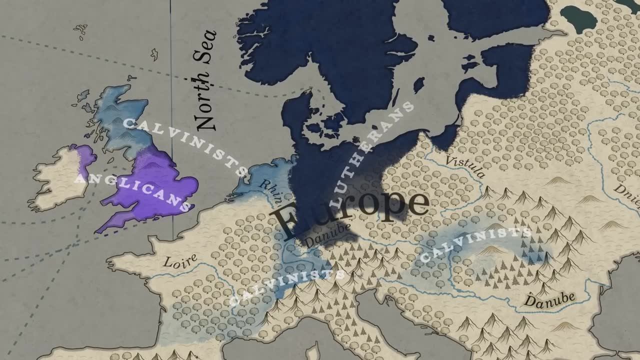 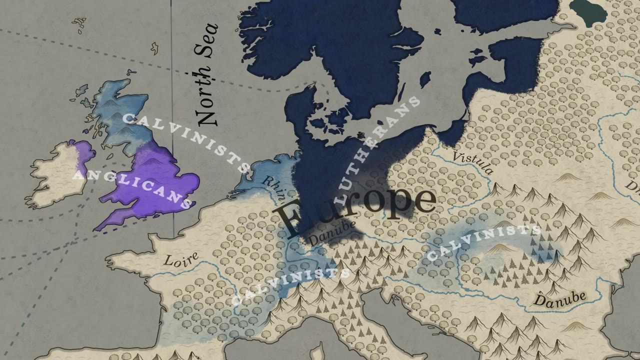 and Protestantism was on an upward path of growth at a fast pace. To combine the spreading Protestant theology, the Roman Inquisition put a heavy focus on the prosecution of anyone deemed a heretic, such as the Protestants themselves. While the Roman Inquisition was drastically milder, 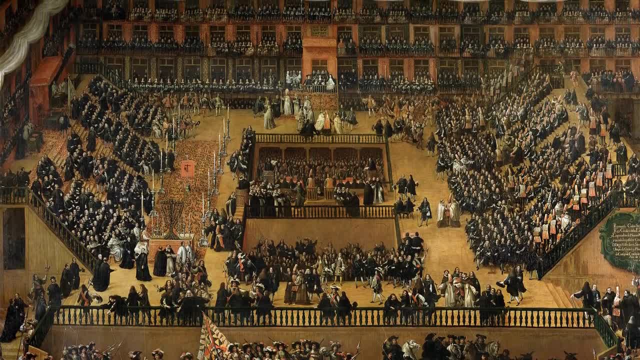 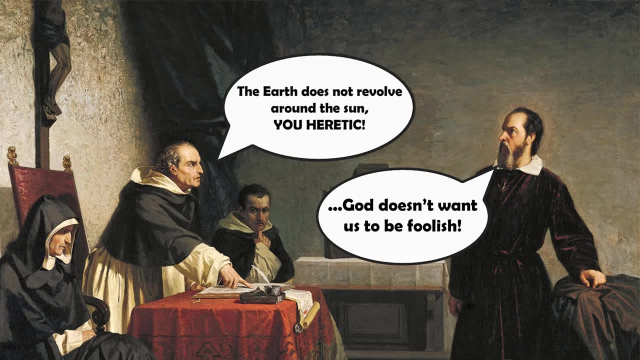 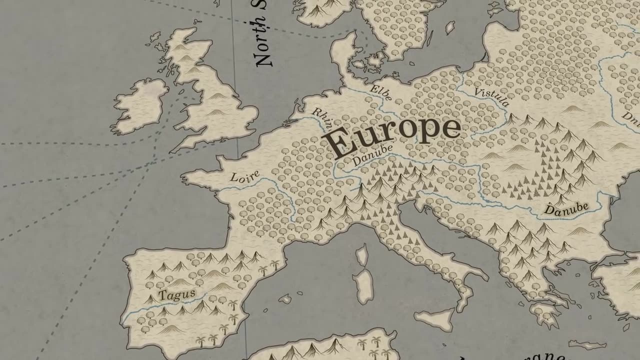 than the previously established Spanish Inquisition. it was famously known for putting Galileo on trial in 1633.. Furthermore, the effects of the Protestant Reformation's popularity triggered wars of religion all throughout Europe, with one of the first being fought in France. 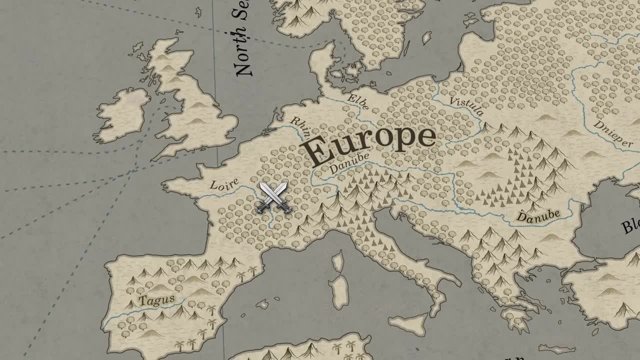 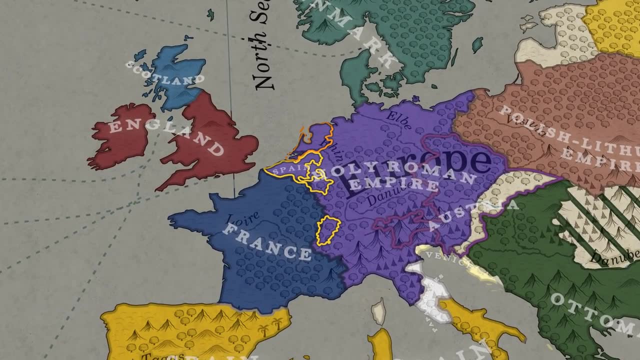 between the Catholics and Protestants and ending in the regaining of France for the Catholic Church, though also providing a level of tolerance for the Protestants in the area. The Thirty Years' War broke out in sixteen, eighteen as well, mainly in the late 18th century. There was a significant increase of war just before that as well. 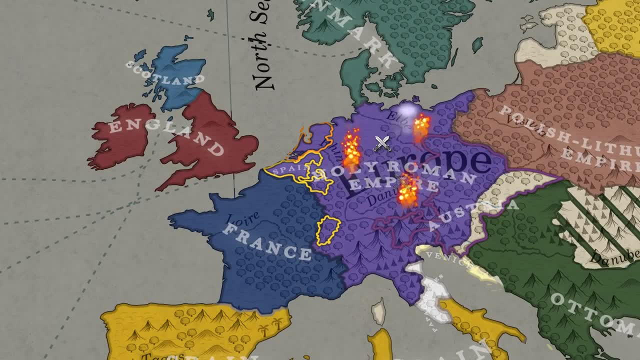 and the second part of World War II was torn on by some French Empire. rif dangitistsawiueller were on alert against a traannonous retrouver of this foreign corridors much rather brutal day. Germany, and is said to have potentially wiped out 40-60% of their population. 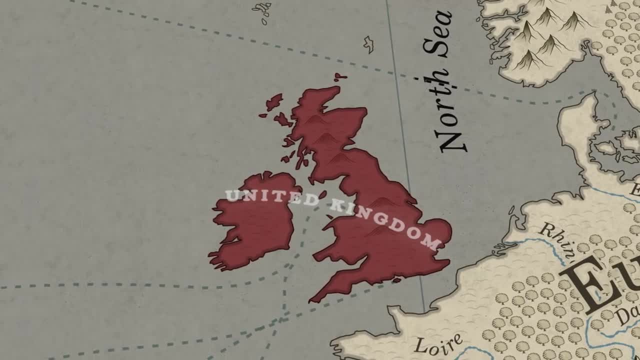 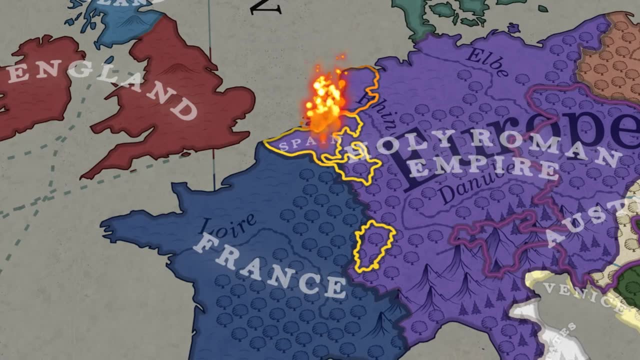 Other wars with Catholic vs Protestants undertones would include the Scottish Jacobite Rising, the Schmalkaldic War, the Dutch Revolt and many more. Even wars that were not solely based on religious conflict were fueled by the disconnect between 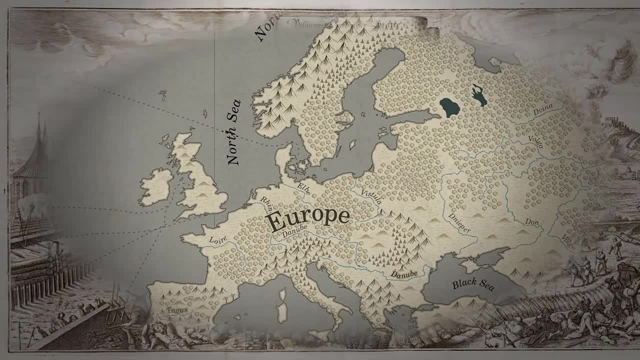 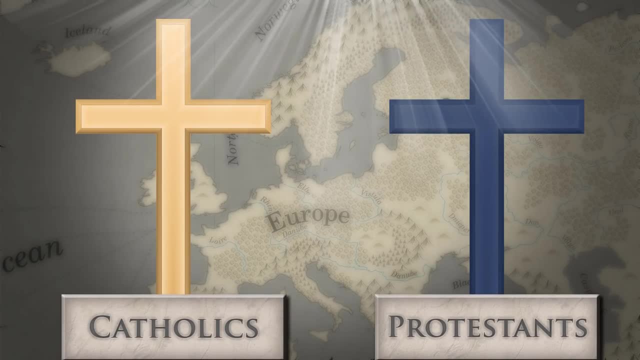 Catholics and Protestants. Today, though the relationship between the Western churches is remarkably better than it once was, There is still a sharply clear schism between the beliefs of Protestants and Catholics, and some disputes and even violence have only recently died down or still remain today. 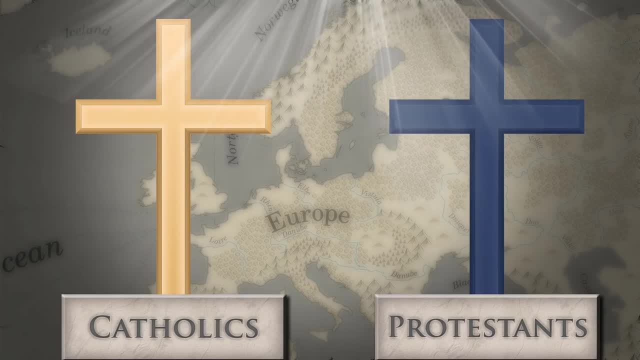 in small pockets of the world. The history and existence of the Protestant Reformation not only stands as a vastly significant event due to its contribution to Christianity. It shows the creation of today's Protestant Christian denominations, but it also shows the true uniqueness of the Catholic denomination which had clearly survived the Great Schism. 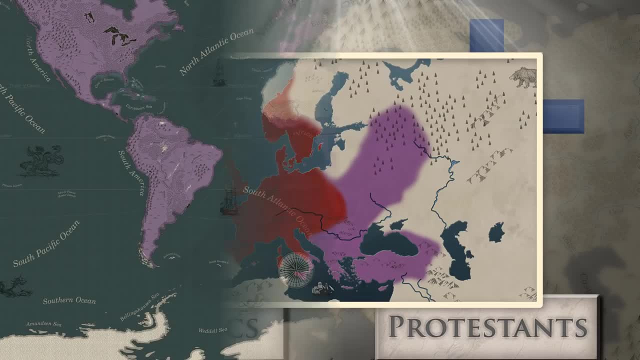 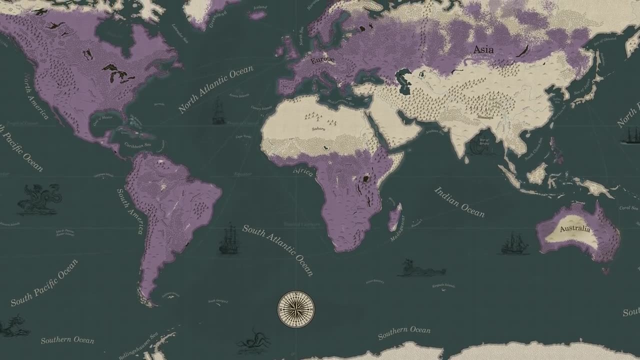 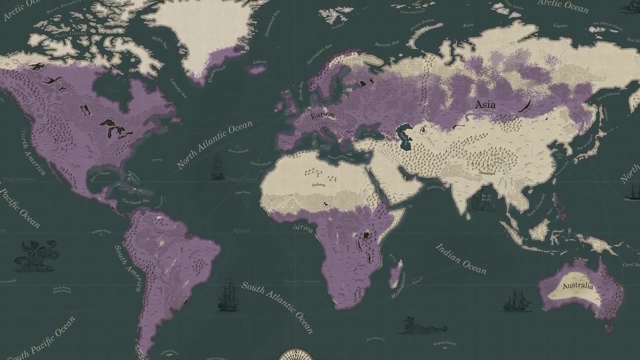 only a few centuries prior. Now, around the world we have thousands of smaller Christian branches or denominations, divided mostly into the Catholic, Orthodox, Protestant, Anglican, Assyrian and Restoration denominations. Undoubtedly, the Protestant Church is one of them. 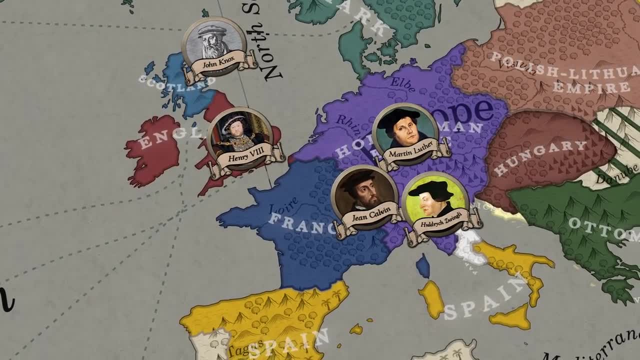 The Protestant Reformation more than helped to shape modern Christianity.